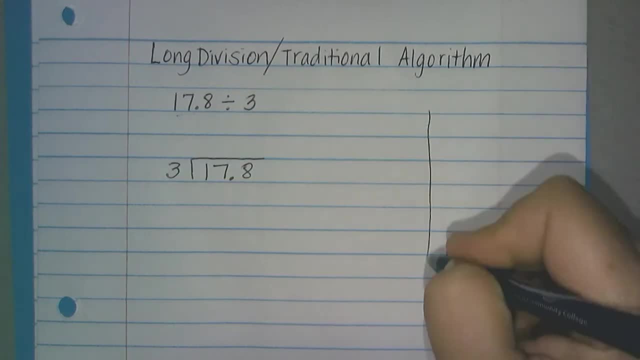 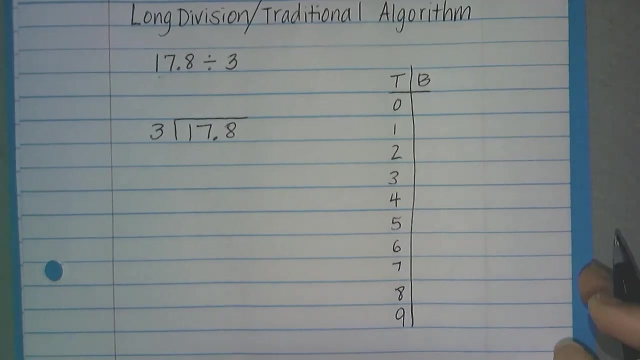 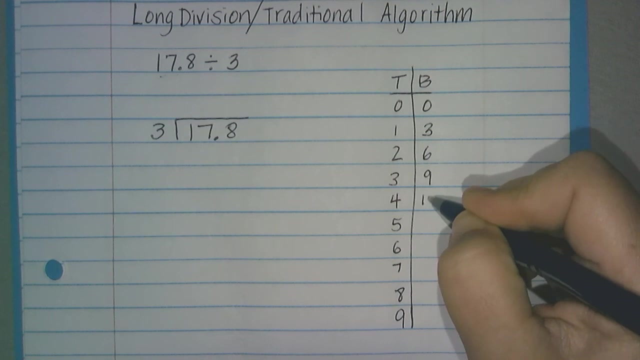 And it also means that 3 is going to be in control of my top and bottom chart, which I discussed in the first video about division Numbering down to 9, and then I have count by threes, because threes in charge 15.. Did you see that calculation? 15. Always double check, 18. And you should. 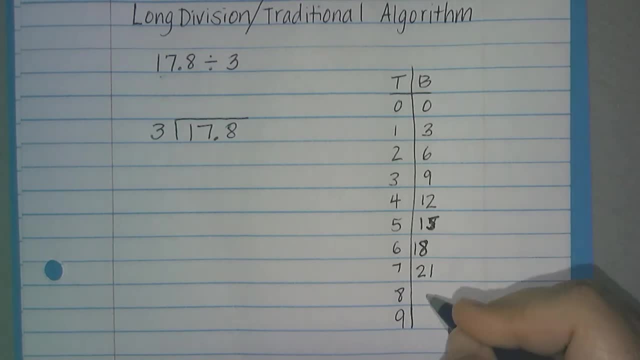 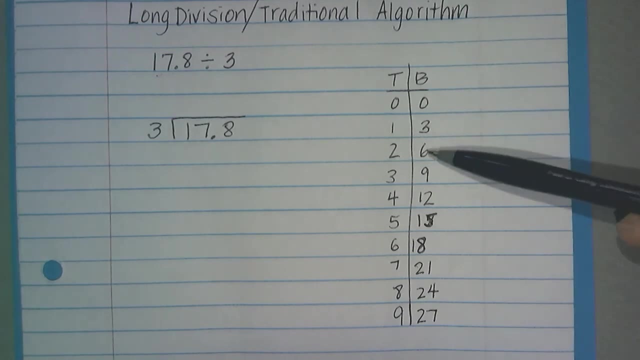 always be doing math and pencil: 18,, 21,, 24,, 27.. 0,, 3,, 6,, 9,, 12,, 15,, 18,, 21,, 24,, 27.. Okay, 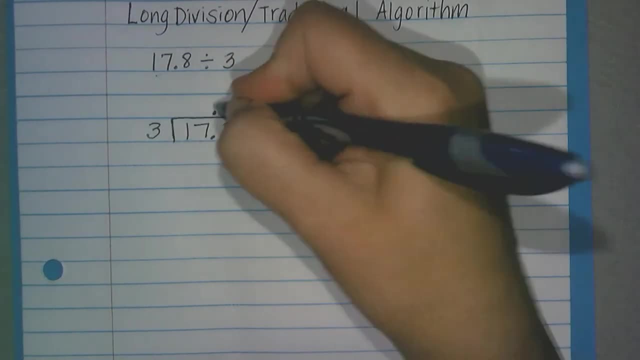 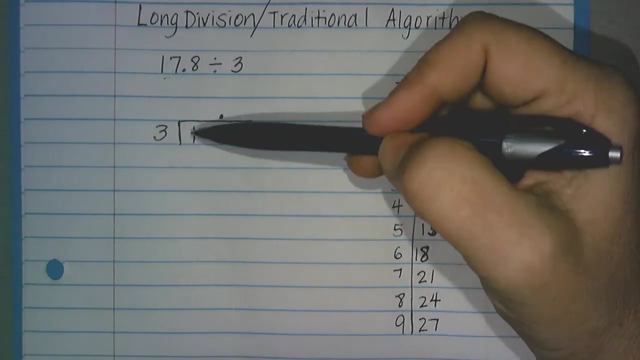 Now I'm going to go over and I'm going to start emptying my truck. after I pop any decimal, I see in the cargo area, pop it up on top of the truck. So I look at it and I say okay, 3 is in the first. 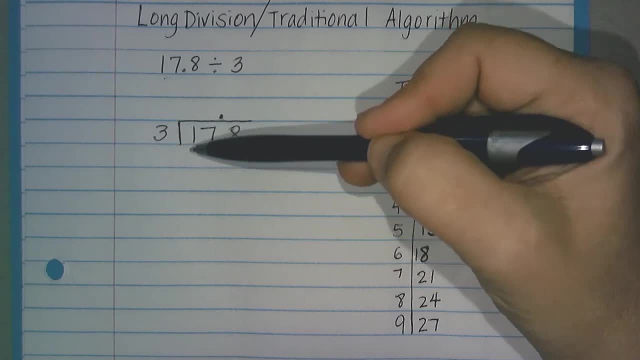 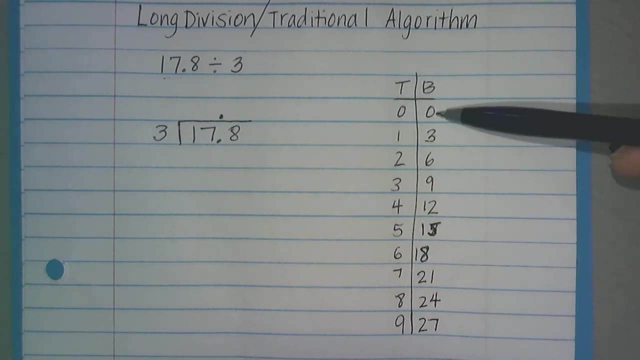 load that I need to empty. So can I subtract 3 from 1, that 1 in the front And I don't see a number small enough to subtract in my bottoms other than 0. So I'm going to follow that step. 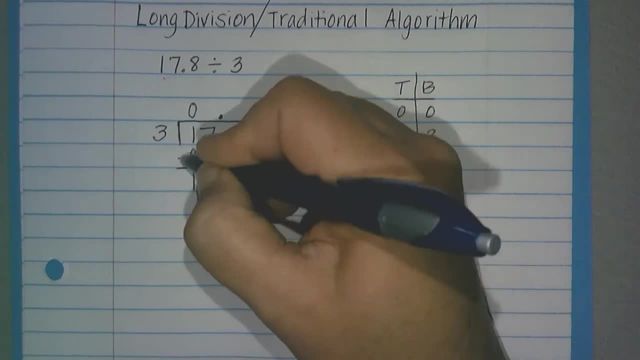 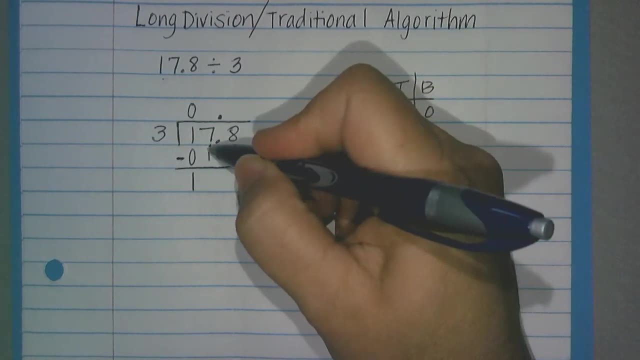 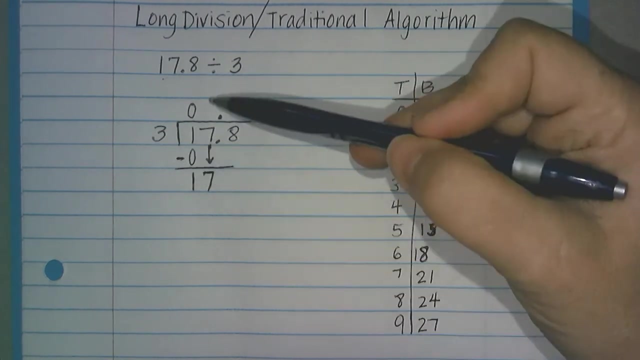 remembering that it's important because I need to remember those 0s later on. Now, the next step in emptying my truck is to drop the 7 down, working one place at a time, because the rules are very strict when emptying cargo. You got to. 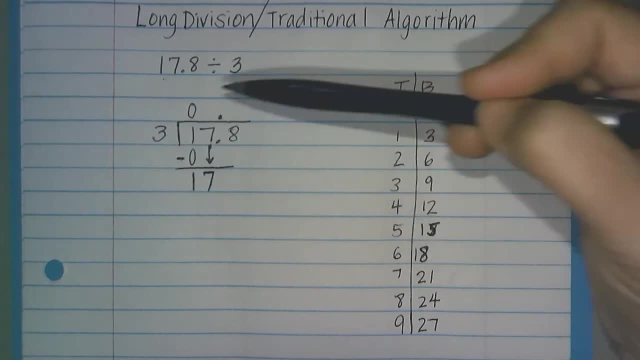 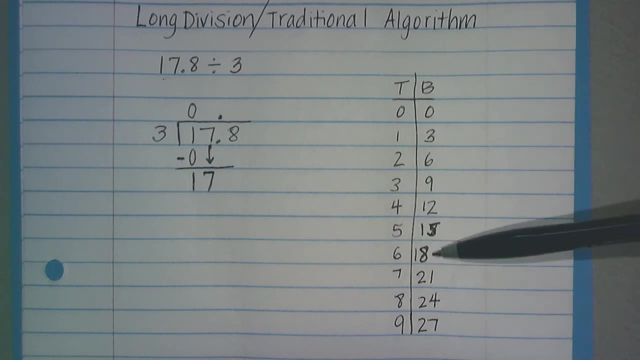 work one digit at a time. So can I subtract any groups of 3 to get this truck unloaded quickly? So I'm going to look over here and say, oh, I can't subtract 18, but I can subtract 15, which is 5 groups of 3.. So 5 is going to go on the top. 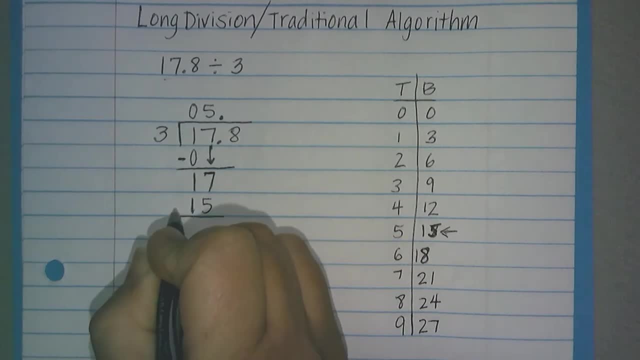 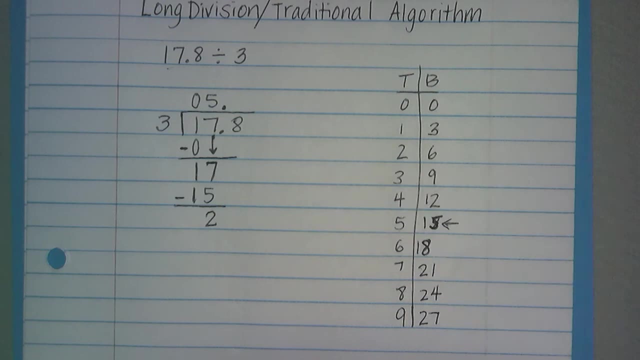 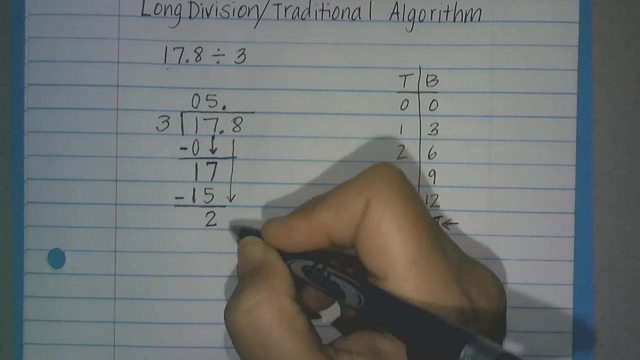 And 15 is my next subtraction problem. 17 minus 15 is 2.. I tap my brain, I say 15,, 16,, 17.. Now my truck is still not empty, So I'm going to drop that 8 down. 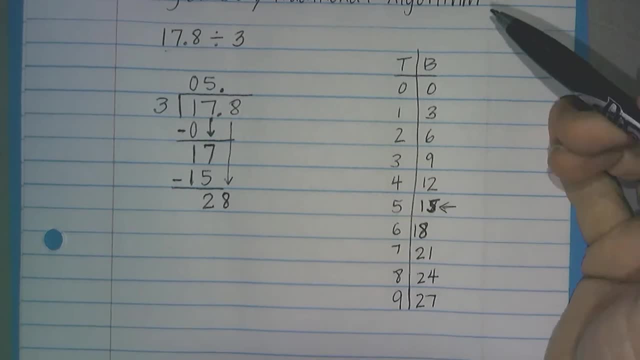 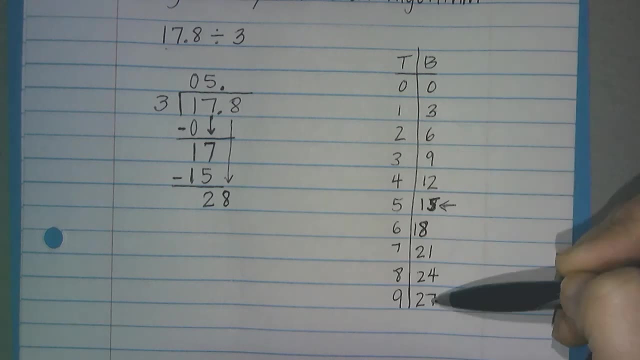 And see: can I subtract anything? how many groups of three can I subtract if I have 28 in there? so I go down 27 and one. another three would be 28, 29, 30, so that would be too big. so I'm gonna subtract 27, which is nine groups of three. so I'm gonna put 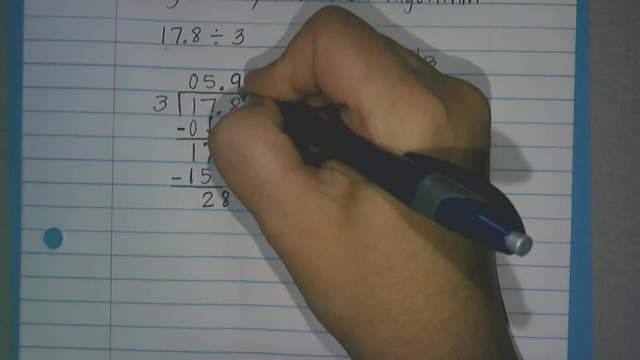 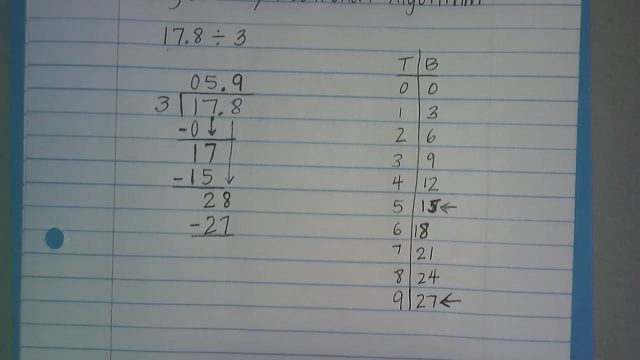 a nine up at the top and I'm gonna subtract 27 and 27 minus 28 is 1. now, in the last video, I told you once upon a time you would use R to show a remainder, but once you are in fifth grade and you're, 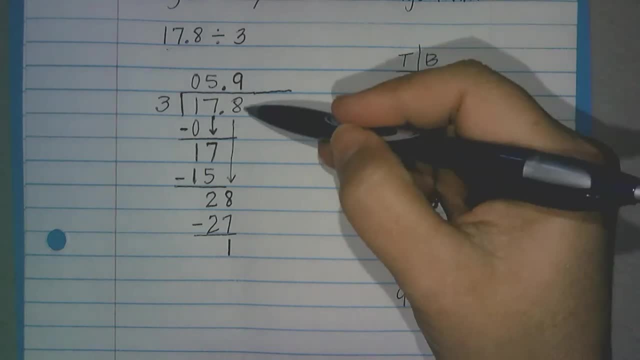 dealing with decimals, the rules change a little bit and I can add as many zeros as I can without changing the value, which is true. because I can add as many zeros as I can without changing the value, which is true. because I can add as many zeros as I can without changing the value, which is true. 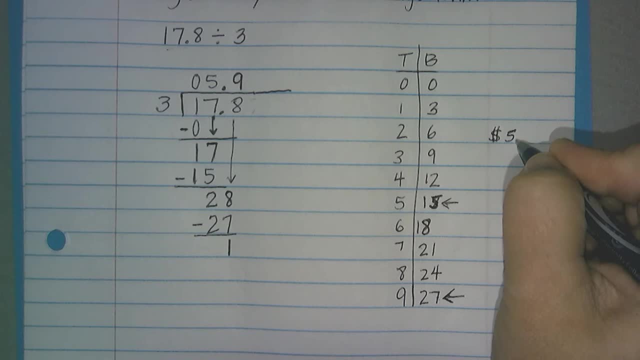 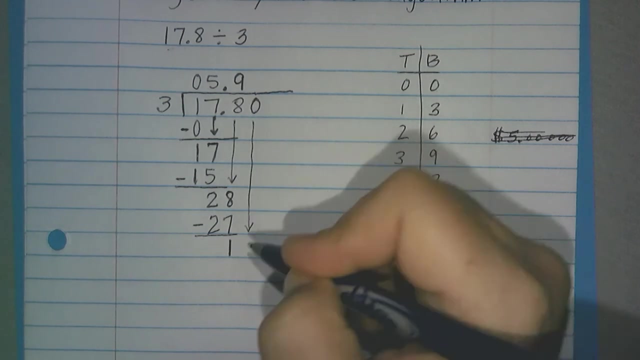 if you think about it, if you had five dollars and there was a decimal here, no matter how many zeros I added, you still have five dollars. that's a decimal. so I can add a zero here and drop that down, and then I'll go over and I say how many. 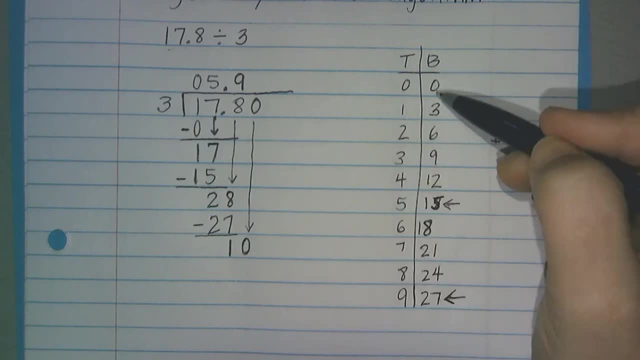 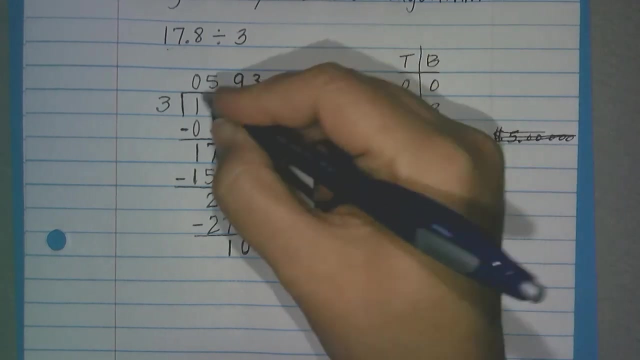 groups of three can I take? there's ten in the truck so I go down and see there's a nine. I can't do twelve so it would be too big. I have ten, so nine and that's three groups of three. so three, using my top and bottom chart, is going to go on the top and nine is going to go on the. 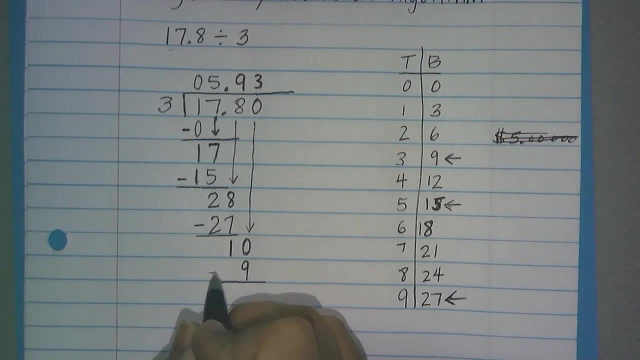 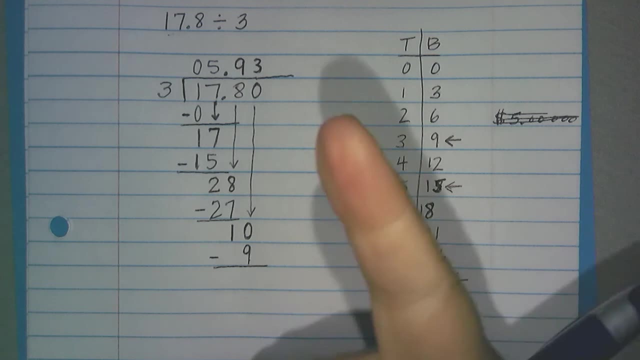 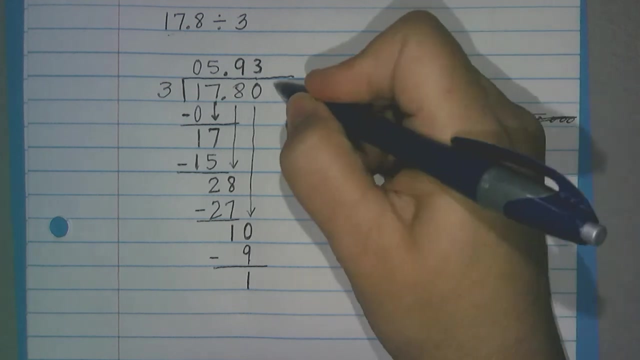 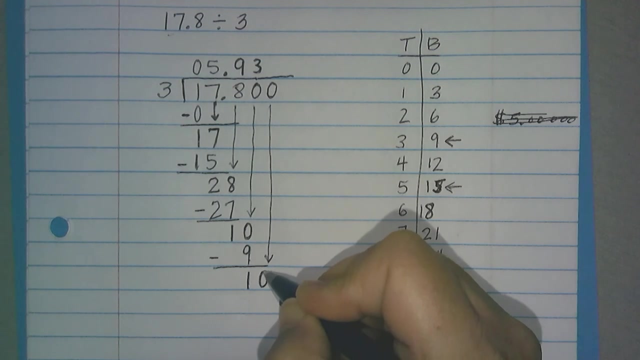 bottom, and then I'm going to subtract and I tap my brain and say nine, ten, it's one away. nine plus one is ten. now I can add another zero, because I can add zeros all day without changing the value. that's why they call this long division, because you end up kind of going along here. now, if I, if you,